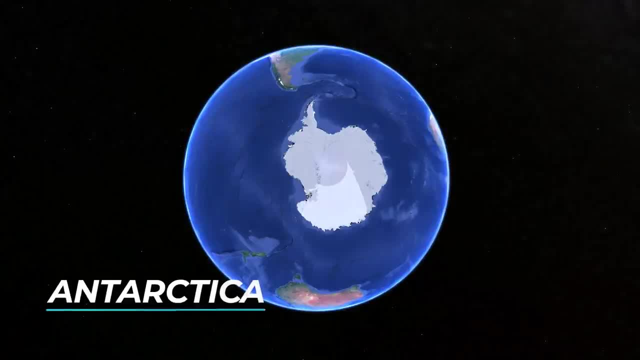 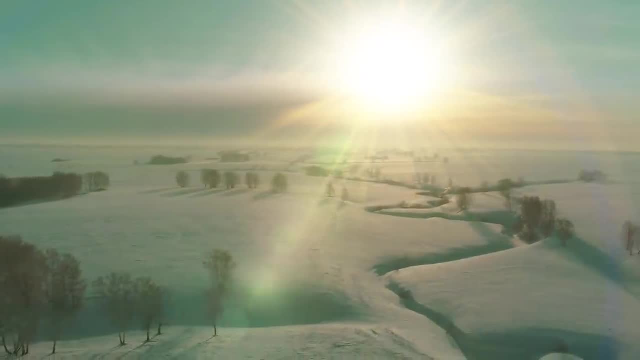 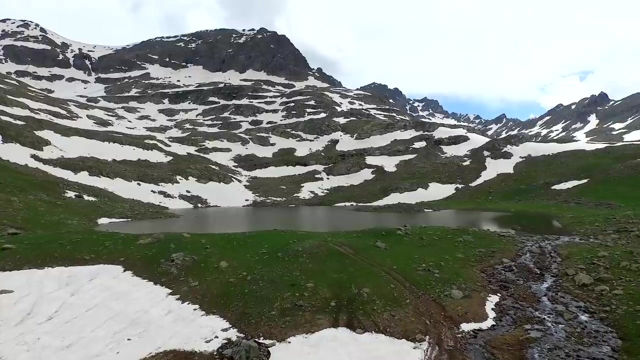 In a region called Antarctica. These climate zones are very cold because the sun does not directly hit these areas. The summers in these regions are not what we think of when we hear the word summer. In fact, they are quite the opposite. Summers in the poles are still very. 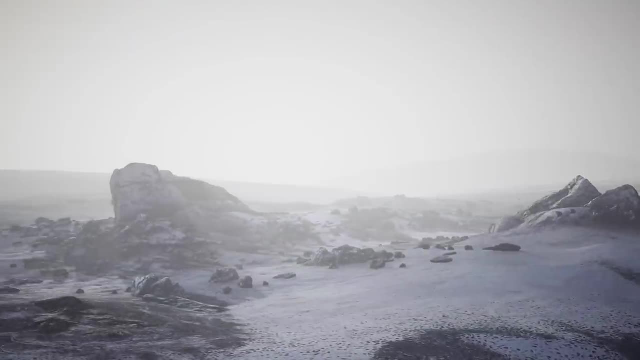 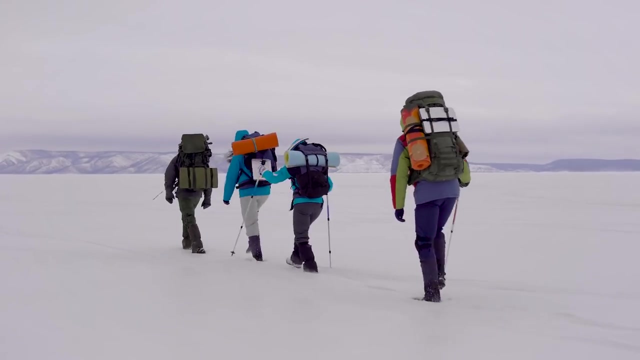 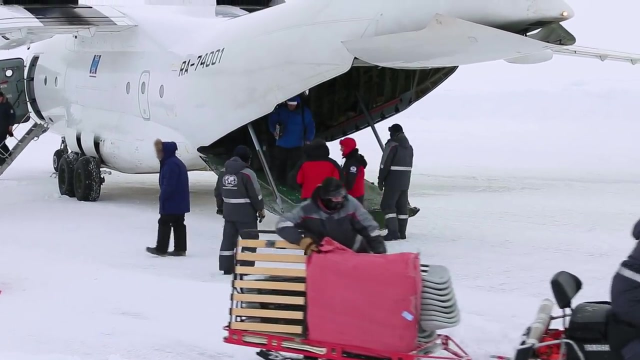 cold. The poles do not support human life. For that reason, there aren't many people who visit the poles, Except for some explorers and scientists who study those areas, And those people wear warm snowsuits that are specifically made for very cold climates. The temperature in the South Pole. 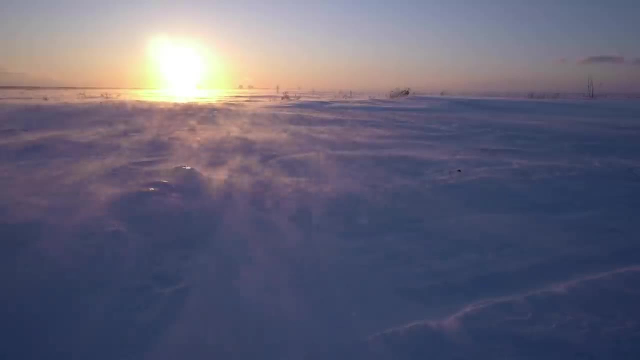 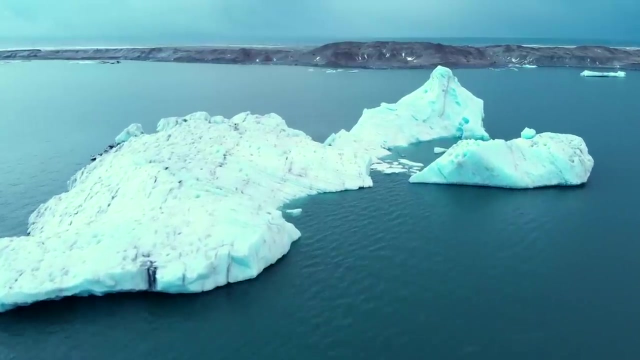 is a lot colder than in the North Pole. In fact, it never gets above freezing in the South Pole, But it does get a bit warmer. in the North Pole The temperature may even go above freezing for a time, When it does some of the ice melts. 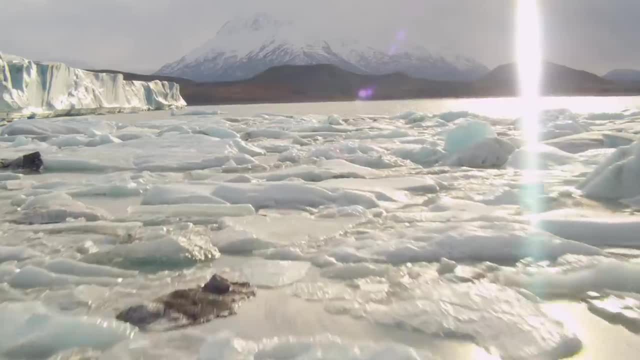 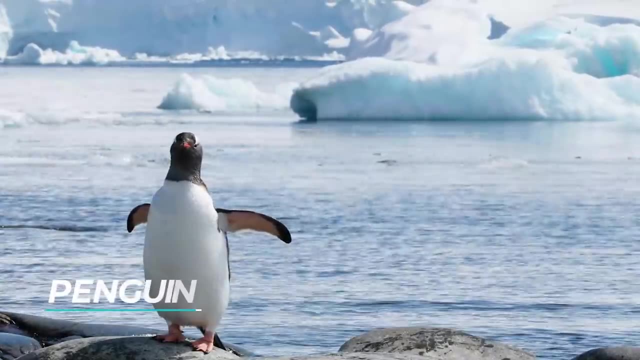 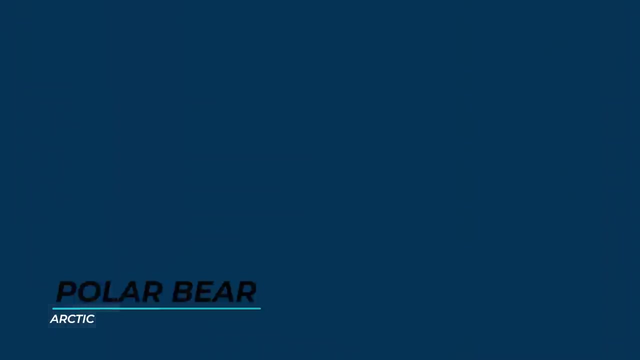 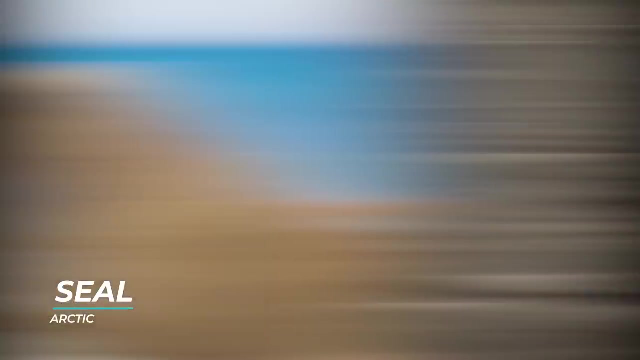 Because the Arctic, or the North Pole, is a bit warmer, it has a wider variety of animal life than the South Pole. Some of the animals found in the Arctic region are penguins, reindeer, orcas, polar bears, Arctic fox, Arctic hares and various seals and walruses In the Antarctica. 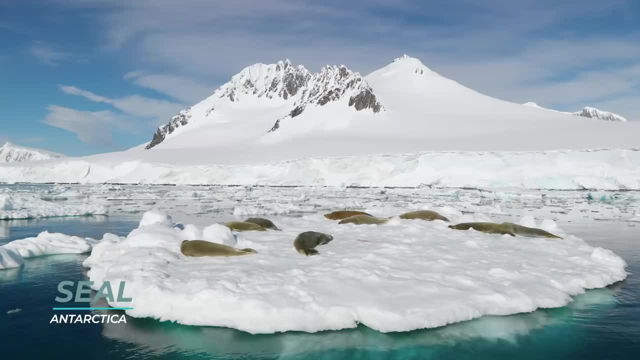 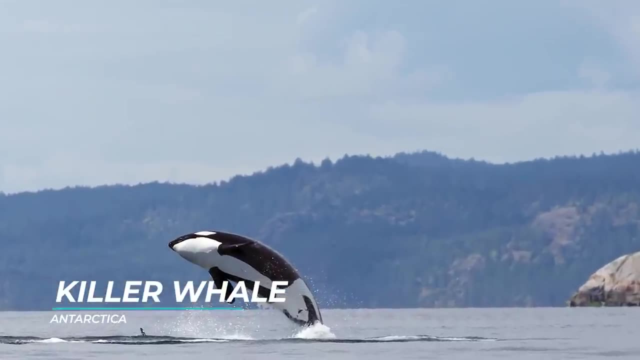 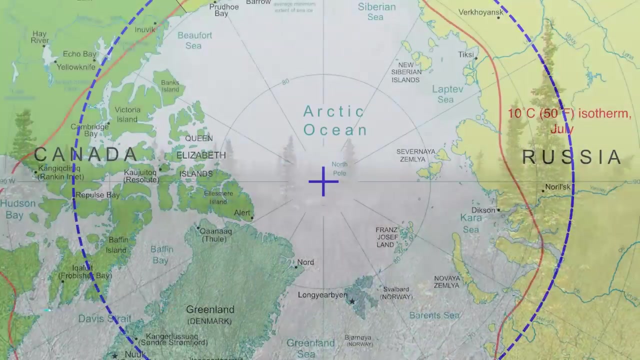 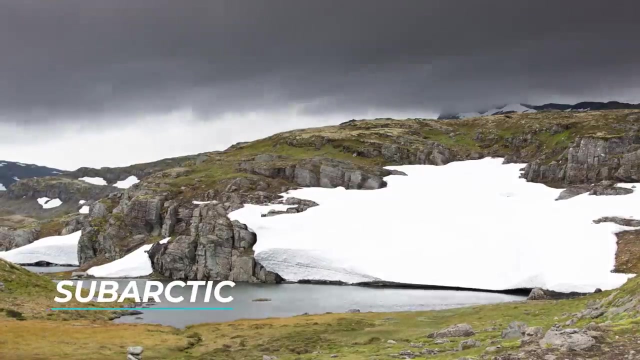 there are various types of penguins, Seals, birds, albatrosses and killer whales. Parts of Canada, Greenland, Iceland, Russia and Alaska are in the Arctic Circle, which is an imaginary line around the North Pole. The area outside of the Arctic Circle is called the 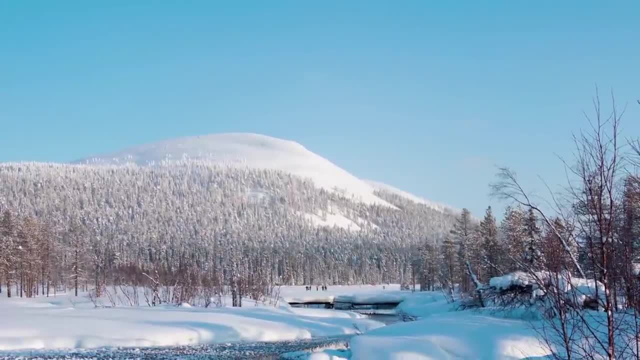 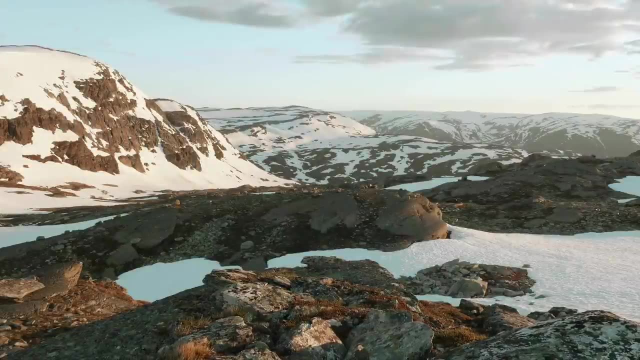 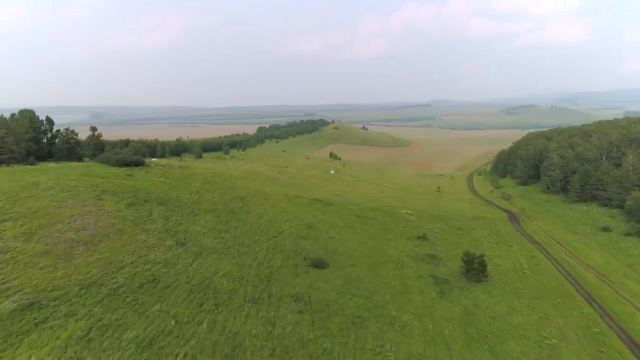 sub-Arctic. Some people do live in these areas, which are further away from the North Pole. It is a bit warmer in these areas, but still colder than almost every other region in the world. Some plants grow in the sub-Arctic. The seasons are very short there. 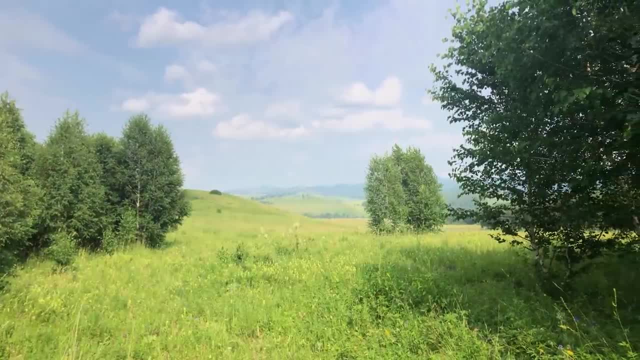 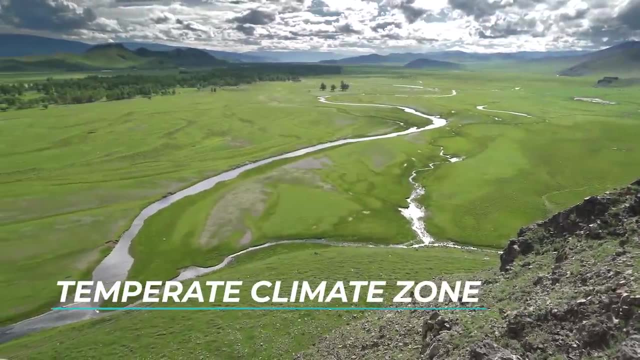 but the daylight hours are very long, so things can grow in a shorter amount of time. The temperate climate zone is an area where the temperatures are mild. In fact, the word temperate means mild or pleasant. Both warm and cold temperatures are mild in the Arctic Circle. The temperature in the Arctic Circle. 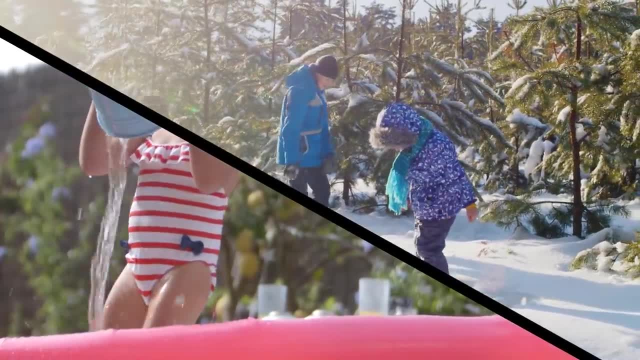 is around 0.6 degrees Fahrenheit. The temperature in the Arctic Circle is about 0.5 degrees Fahrenheit. The most warm and cold climates exist in the temperate climate zone. In the warm climates, the winters are mild and wet and the summers are hot and dry. 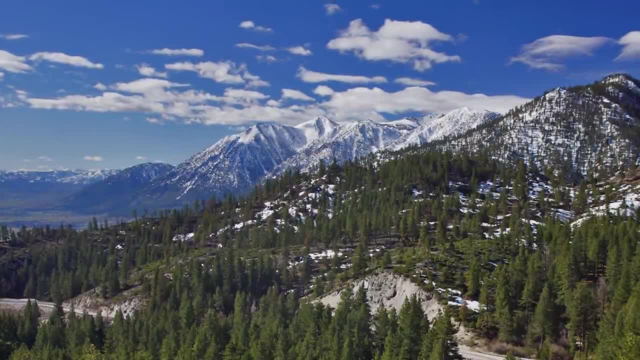 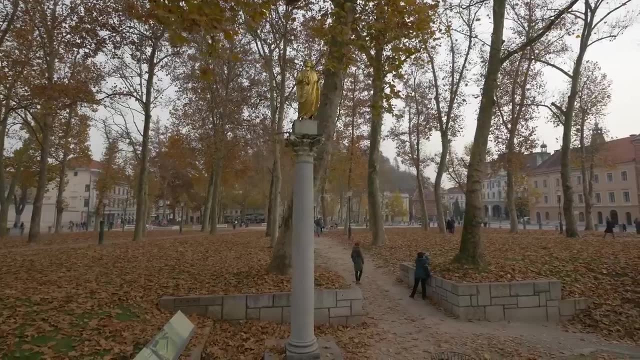 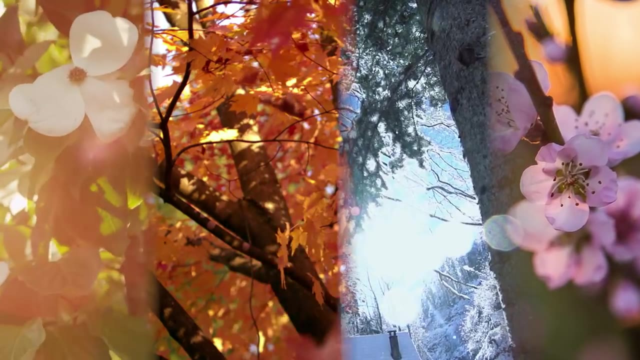 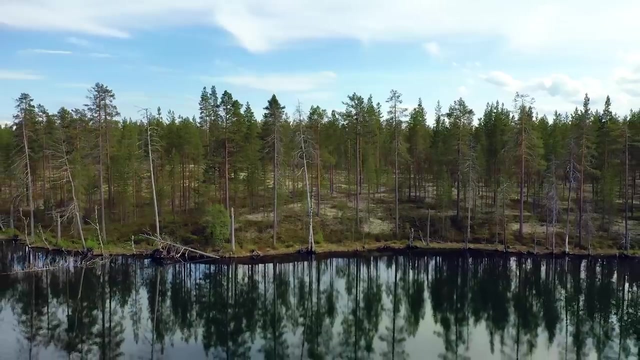 In the cool climates the winters are cold, with snow and freezing temperatures, but the summers are warm. There are four seasons in temperate climate zones: fall, winter, spring and summer. A lot of the United States, Europe and the southern half of South America fall within this climate zone. 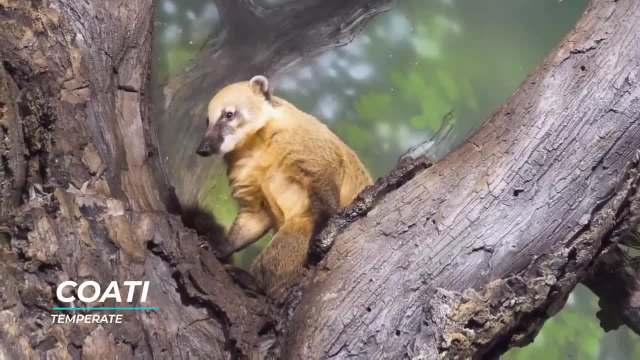 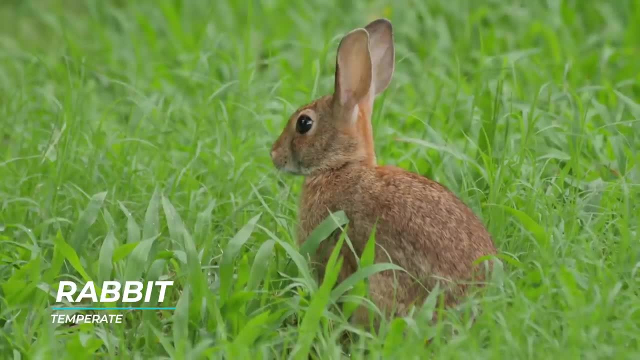 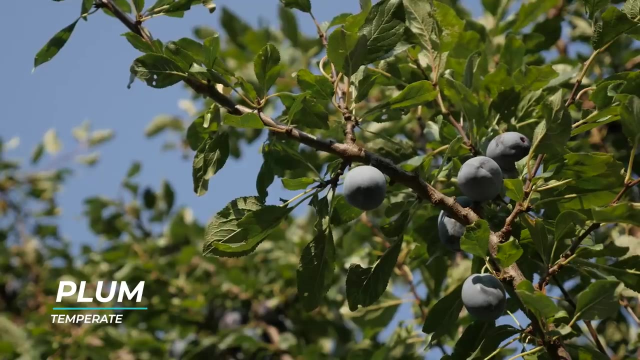 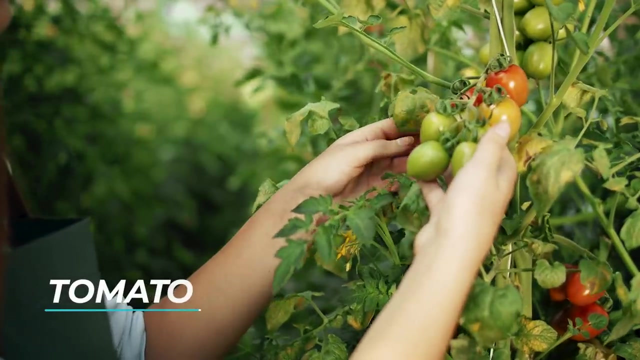 Many different animals live in this zone, including bears, lions, deer, mice, rabbits, snakes and more. Fruits like peaches, apples, plums and strawberries grow in temperate climate zones, as well as vegetables like tomatoes, corn, wheat, potatoes and onions. 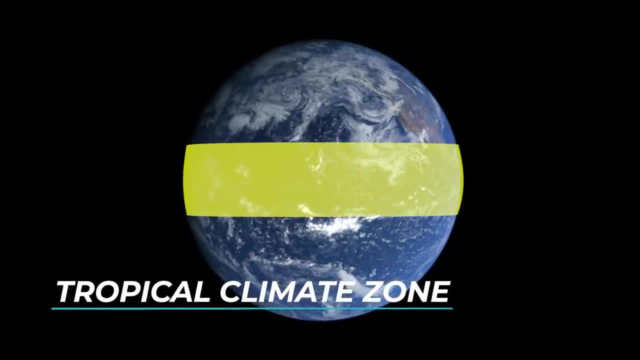 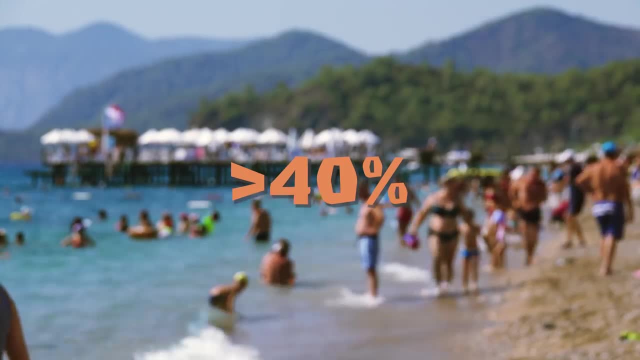 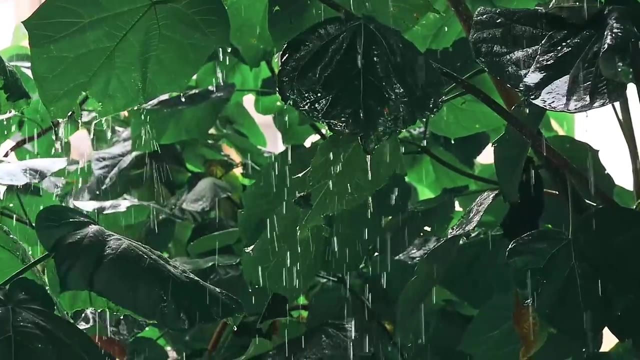 The tropical climate zone is just north and south of the equator. More than 40% of the people on Earth live in this climate zone. The temperatures are very warm in these regions, so it can get pretty hot. Tropical climate zones get a lot of rain. especially in the summer. In the summertime, which makes it very humid. that humidity can make you feel even hotter. In wintertime there is less rain than in the summer, but it still stays warm. The Congo in West Africa and the Amazon in Brazil are both rainforests and examples of tropical climates. Thousands of islands like Kauai, Bora Bora and Tahiti are also located in tropical climates. Unlike temperature climates that have four seasons, tropical climates have very little seasonal changes. Instead, it stays warm all year long, which means that things can grow all year long in. 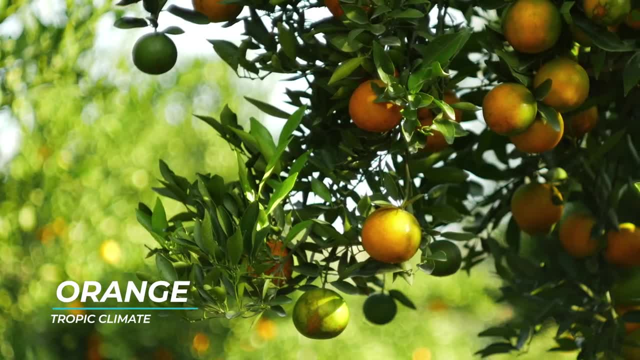 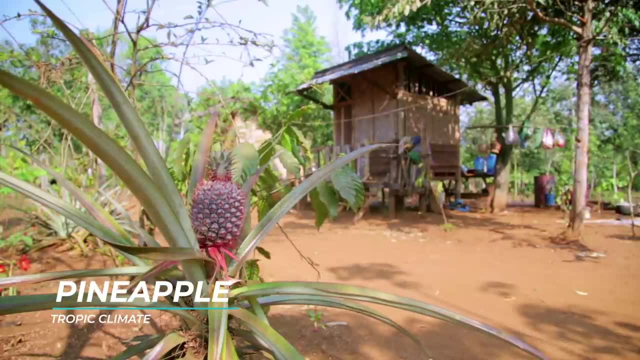 these climates. Bananas, oranges, lemons, limes and pineapples are all popular fruits that grow in tropical climates. Tropical climates have the most tropical climate zones in the world. Tropical climates have the most diverse animals and plants in the world. 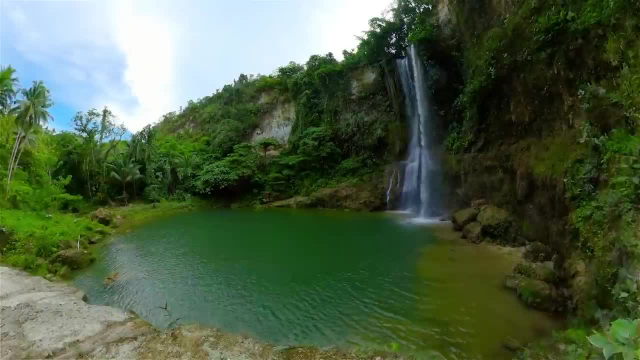 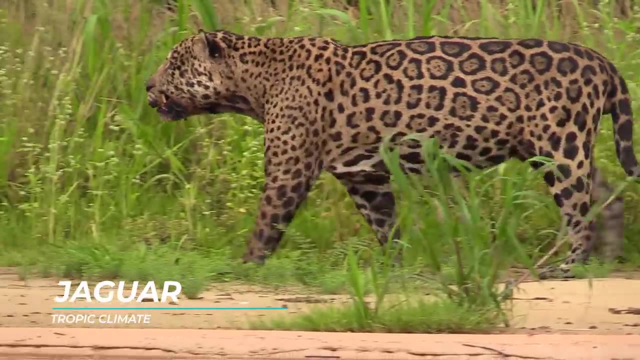 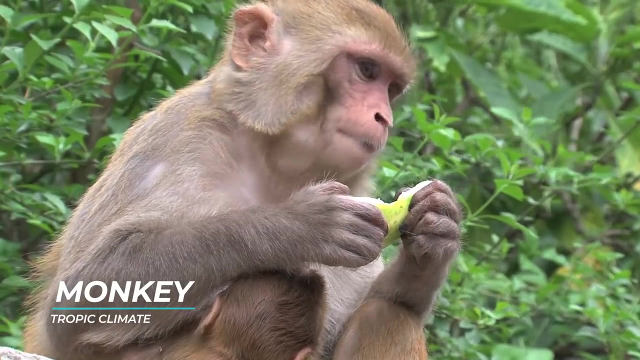 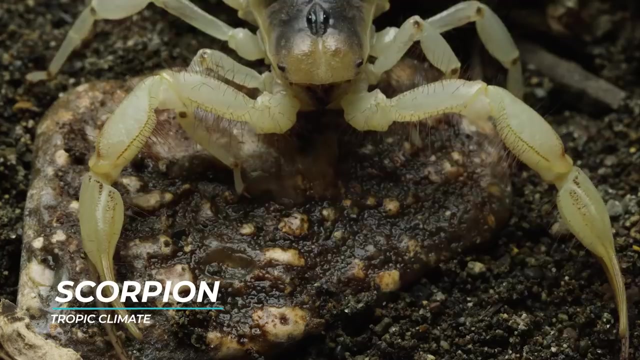 In fact, most of our animal and plant species come from tropical climates. Some animals that live in tropical climates include jaguars, gorillas, toucans, sloths, monkeys and macaws, Many invertebrates like butterflies, centipedes, scorpions. 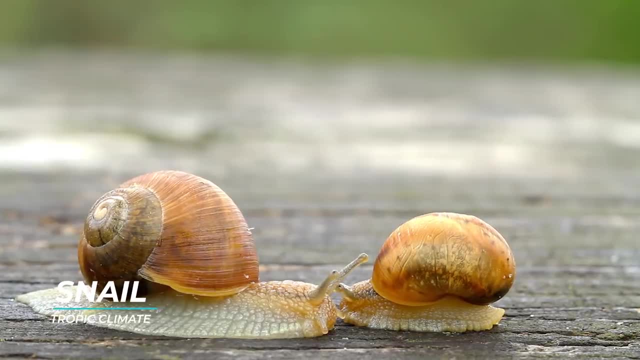 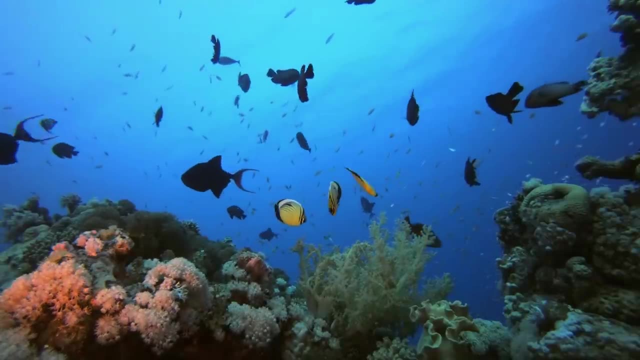 spiders. apes and spiders look very similar to tropical climates. Plenty of Bachelor's Degrees of Tropical Climates include animals which are close to tropical climates. Spiders, snails and beetles are found in tropical climates. There are also many freshwater and saltwater fish in tropical regions that are near the water. 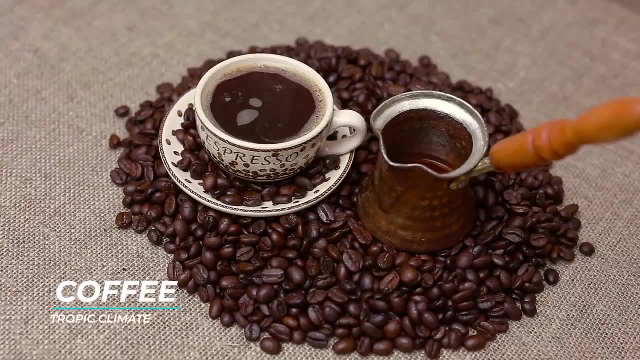 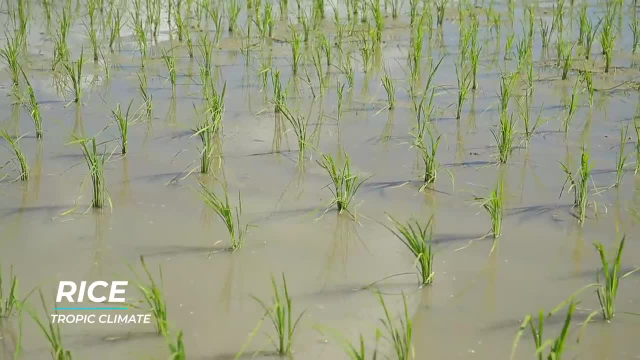 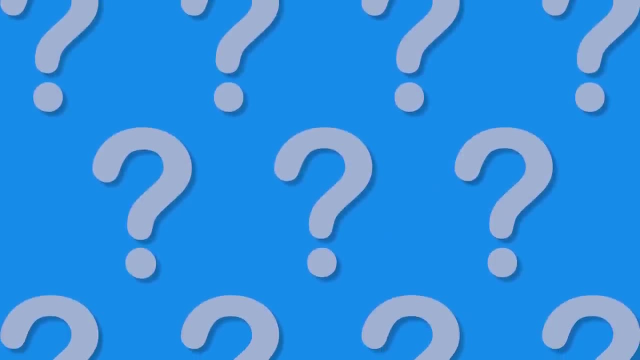 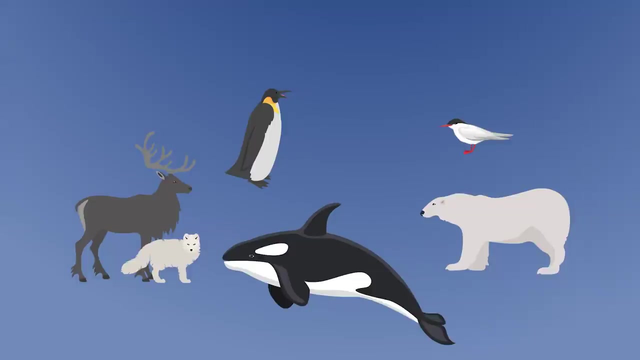 A lot of well-known foods like coffee, chocolate, sugar, vanilla and rice grow in tropical climate zones. Now that you have learned about these three climate zones, let's see if you can answer some questions about each of them. In which climate zone would you most likely find these animals? 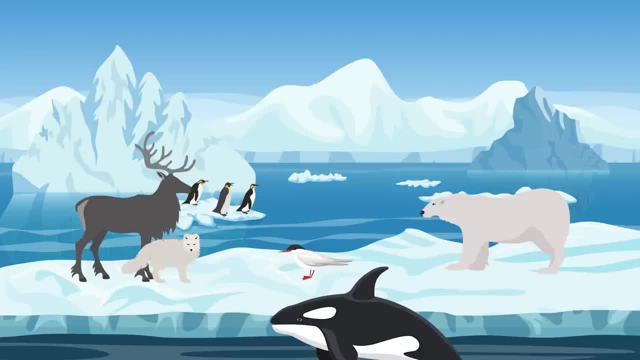 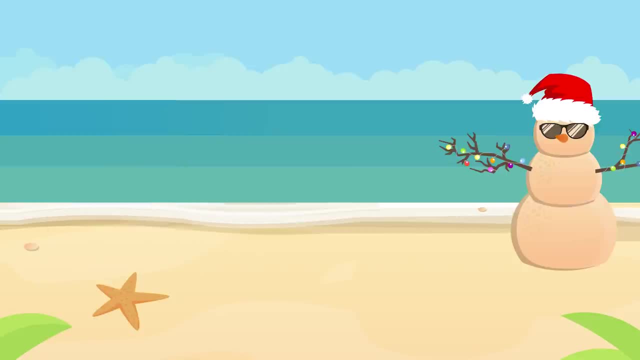 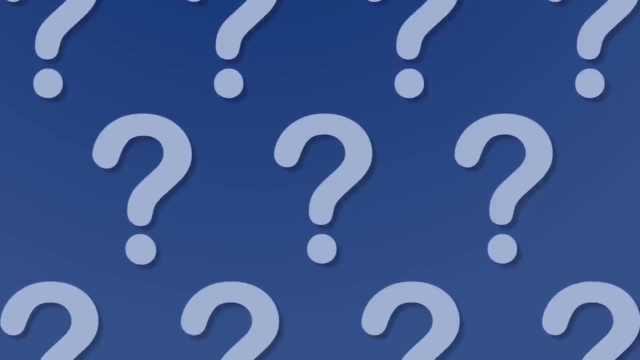 Did you say the polar climate zone? Good job. Have you ever seen a reindeer at the beach? Probably not, And if you have, you might want to call Santa and let him know that Rudolph's taking a vacation. Let's try another one. Which climate zone would these animals live in? 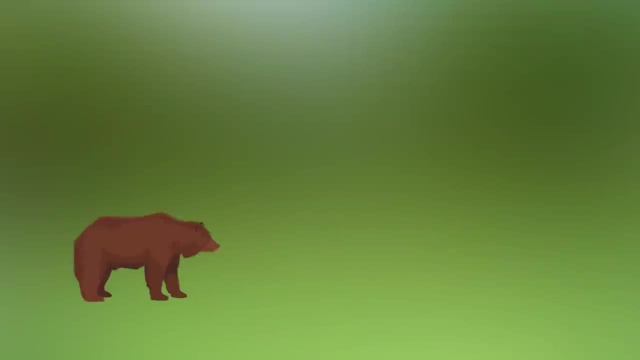 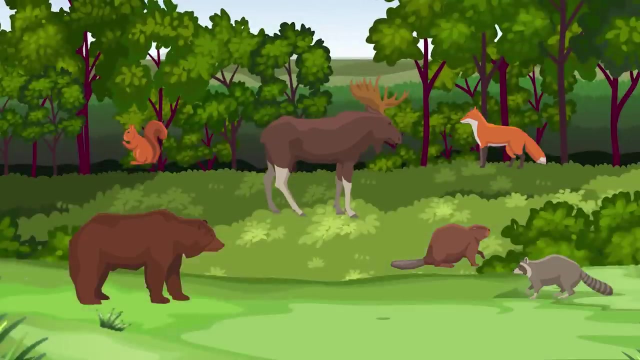 It's the tropical zone, isn't it? Now, which of these three climate zones would you most likely find? Which of these animals do you think you'd find in a temperate climate? If you said all of the above, well done. 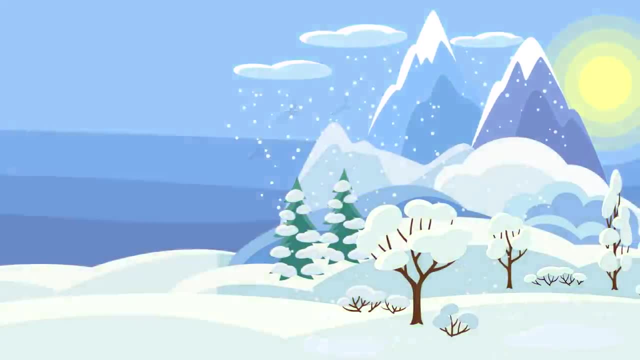 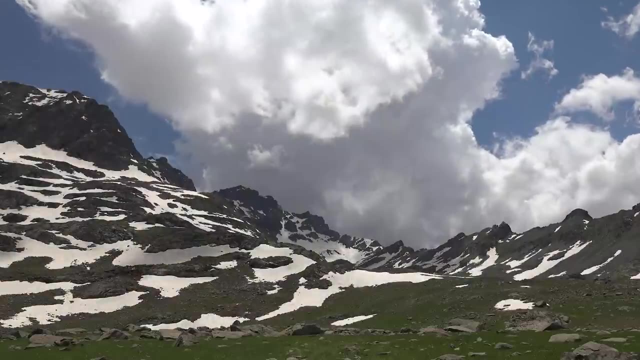 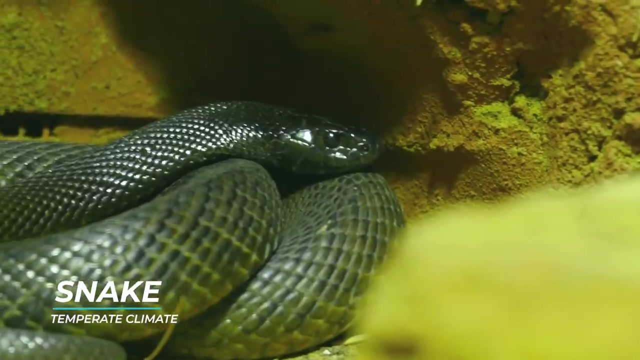 Remember that in a temperate climate, it gets both warm and cold. Animals like white-tailed deer, bison and moose are found in colder regions or higher up in the mountains, While others like turtles, snakes, seagulls and coyotes are found in the warmer climates near the oceans and deserts. 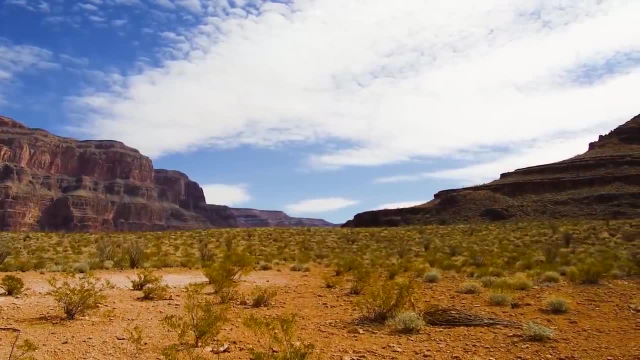 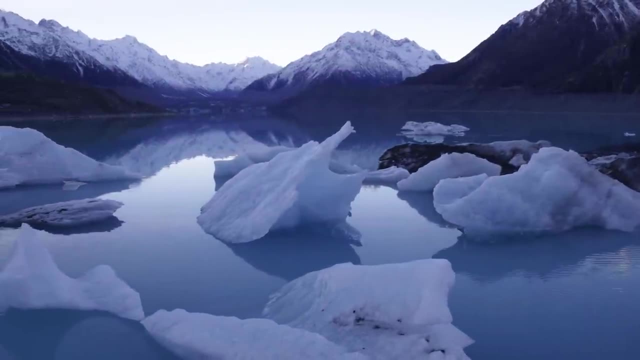 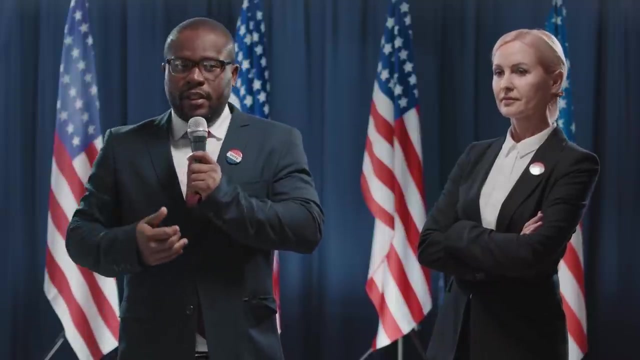 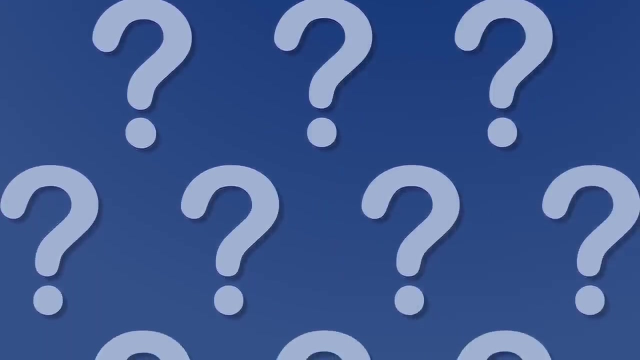 And many more animals can be found in between those two locations. Ready for a few more questions, How might someone dress in a polar climate? Would you wear a swimsuit, a snowsuit or a business suit? I guess a scientist could wear a business suit if she wanted. 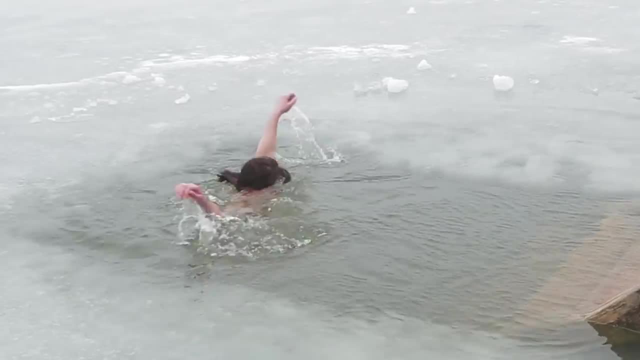 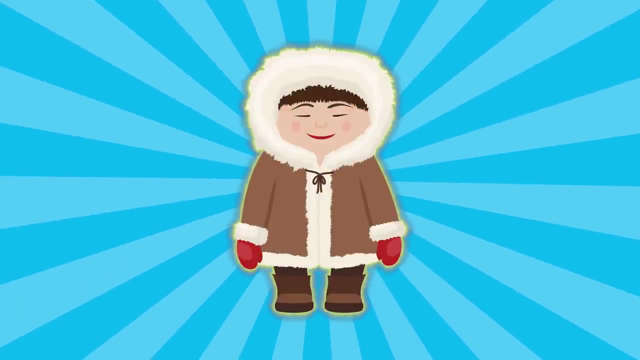 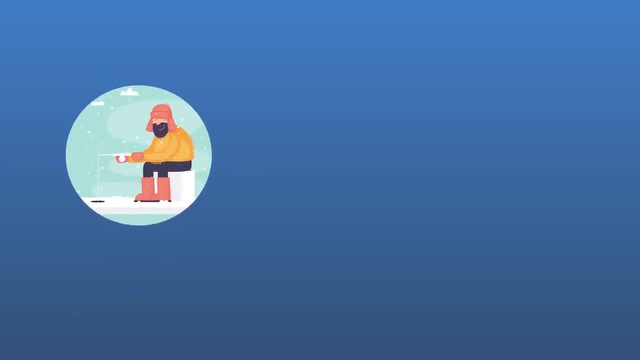 But she'd probably freeze, And she'd definitely freeze in a swimming suit, So a snowsuit is the correct answer. Which of these jobs could someone have in a tropical climate? You probably wouldn't make much money teaching people how to ice fish in a tropical climate.